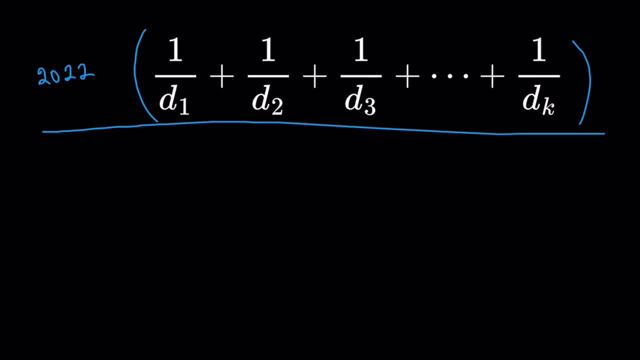 we can't just multiply by 2022.. So we have to divide this result by 2022.. Now take a look at the numerator here. We know that if I expand it out, the first term is going to be 2022 divided. 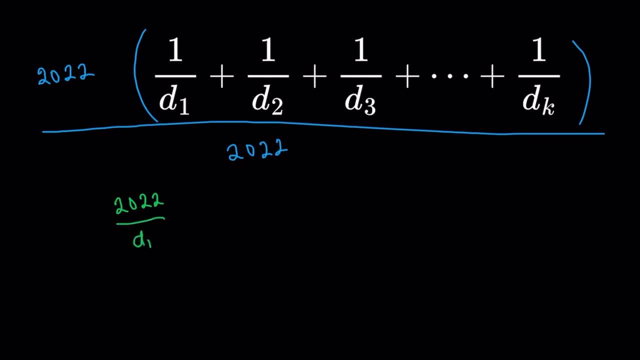 by d1.. Now we know d1 is a factor of 2022. So we know that 2022 divided by d1, that's going to be a divisor of 2022. We could have the same reasoning for 2022 divided by d2.. That's going. 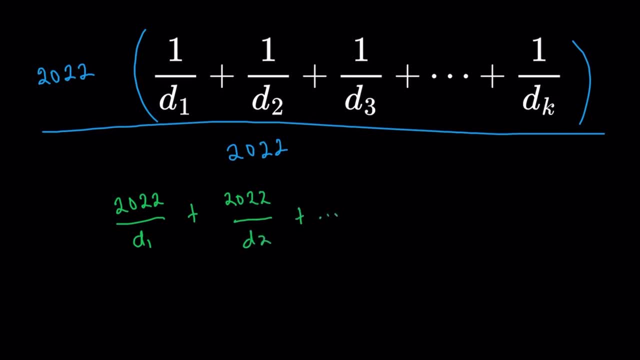 to be a factor of 2022. And this will continue all the way until the last term. 2022 divided by d sub k- In fact, we could try to get what k is. So we know that 2022 in factored form. 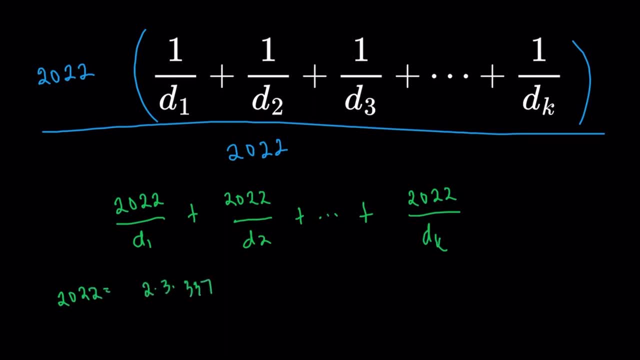 that's going to be 2 times 3 times 337.. So using the counting the number of divisors trick, we could just kind of say that okay, the exponents are ones and we just have to add one to each of the exponents, So it becomes 2,, 2, and 2, and finally multiply them out. 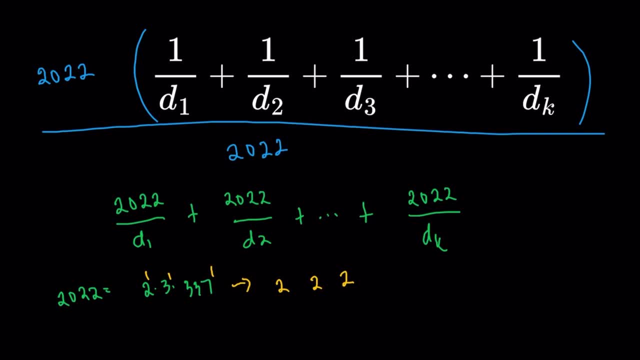 So here, 2022 has eight divisors, So that's going to give us the value of k. So let me just write this one a little bit more specifically: d sub k, it's going to be d sub 8.. All right Now. 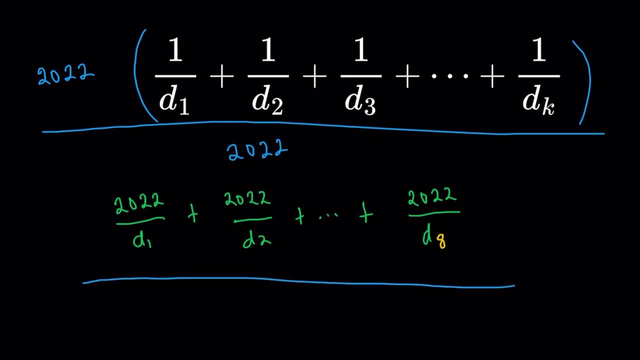 as I've mentioned, the numerator here are just sum of divisors. So we know that this one is a divisor. This one is a divisor all the way until d sub 8.. That's a divisor. But obviously d sub 1, d sub 2, all the way until d sub 8, they are different numbers. 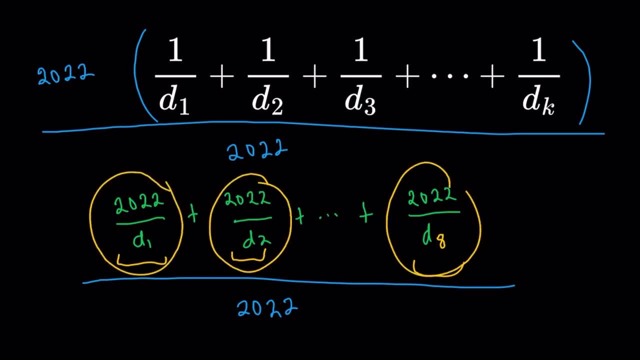 So these eight numbers over here are the divisors of 2022. So essentially, the numerator. here it's just the same as saying we're asked to get the sum of the divisors of 2022.. All right, So it's simple as that. We just have to realize this trick, that, oh, since we're just 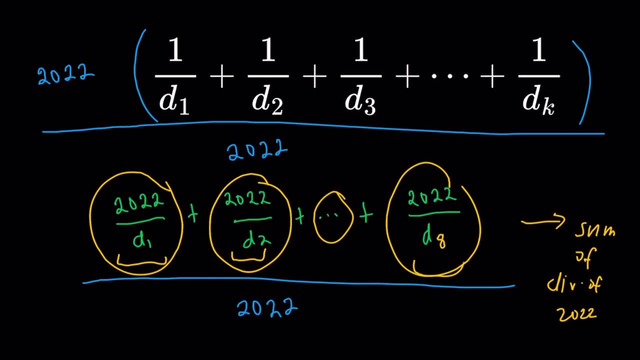 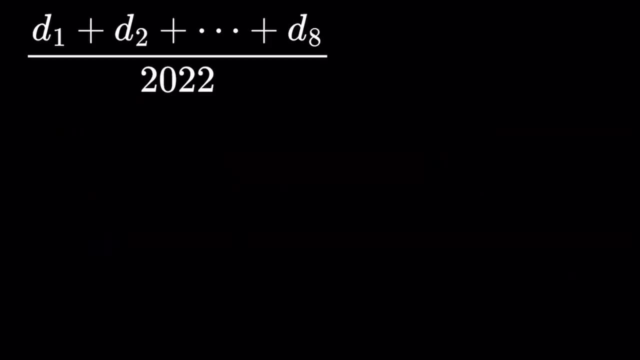 adding factors, then it must be the same thing as just getting the sum of the divisors of 2022.. And, yes, we have this expression to be equivalent to the previous one, All right. So now that we have this, we now realize that. okay, the trick for getting the sum of the reciprocals is apparently: